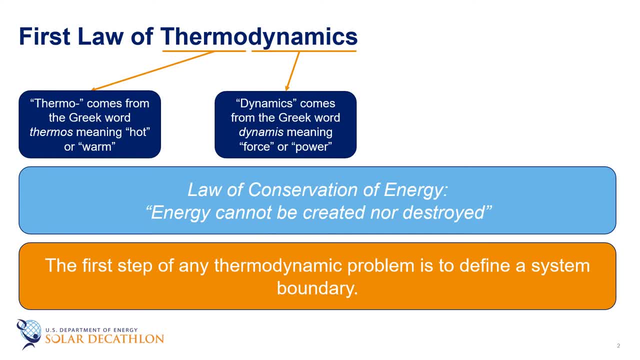 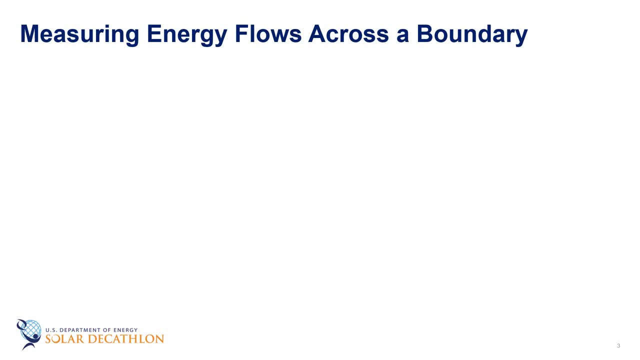 first step of any thermodynamic problem. Without a boundary, we cannot track the transfers. After defining this boundary, the next step is to identify the different energy flows that cross the boundary. In general, we look at three major types of energy flows: work, heat and the energy associated with mass crossing the boundary. Heat and work are: 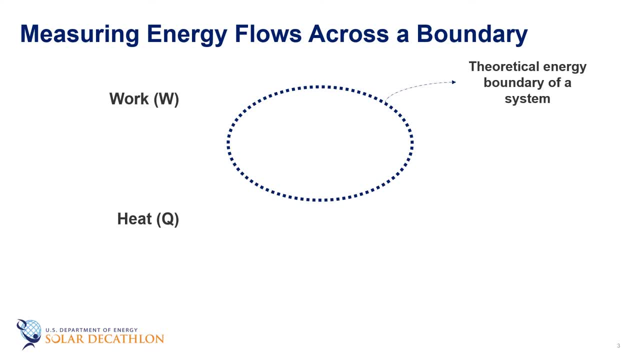 different ways of transferring energy across the boundary. From the building science point of view, heat is the transfer of thermal energy across the boundary because of a temperature difference at the boundary, and work is the transfer of mechanical or electrical energy across the boundary. So a power line crossing the boundary into a building is considered electrical work entering the building. 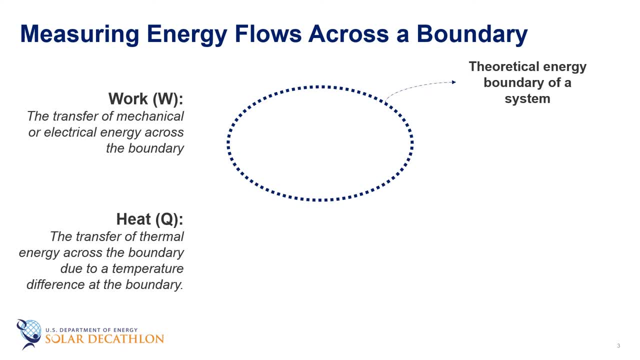 Energy being lost from a warm building in the winter to the cold surroundings is heat. Well, what about a natural gas pipeline that enters the building for the furnace and for cooking? Is that heat or work? This one is actually the energy associated with the mass of natural grass crossing the boundary. 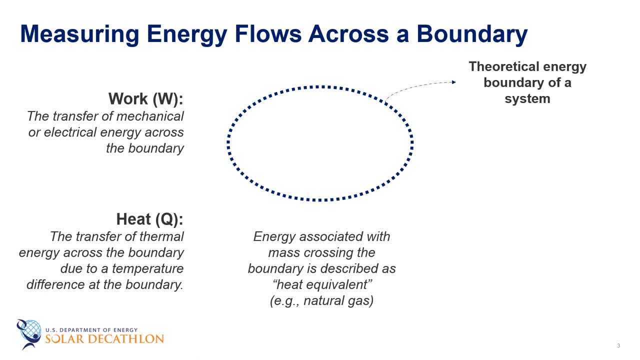 However, for simplicity, we can think of that as an equivalent amount of heat that is crossing that boundary. We symbolize work with a W and heat with a Q, and that represents the energy that has crossed the boundary. When I add energy to a system, that has to be equal to the change of energy of that system. 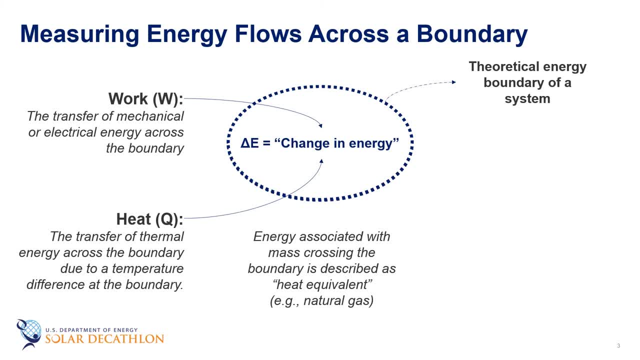 However we show the change of energy, We see the change of energy as the change of E. So in this simplified version of the first law of thermodynamics we can look at work plus the heat going in has to be equal to the change of energy within that system or within that control volume. 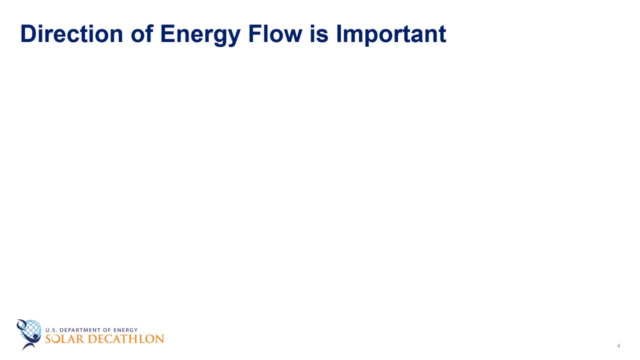 One thing to note is that the direction of flow is important. So we'll draw another system here and we'll say we've got some mechanical work and some electrical work going into the system, And then maybe we also have some electrical work going into the system. 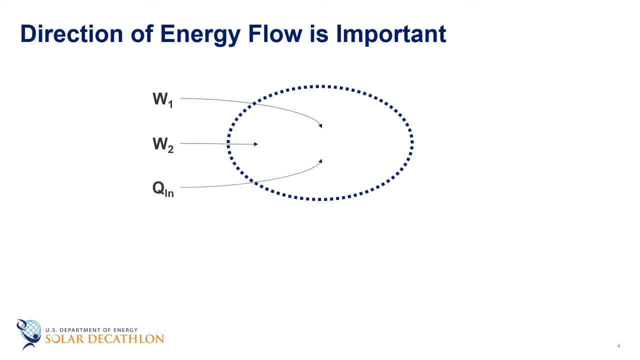 We have some heat that's going into it. That could be represented, in our case, by the energy content in a certain type of fuel, such as propane or maybe natural gas, And so then we might also have some heat that is being lost from the system. 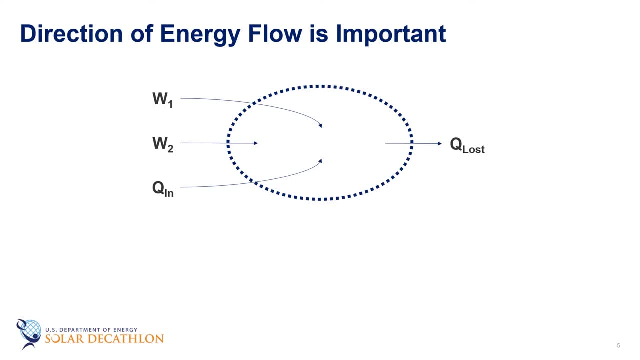 We'll call that Q lost. We need to go through and add up all those different flows that are going in and out, And we do that by drawing the energy flows across the boundary. Basically, we show that as arrows going in, as positive, and arrows out are negative. 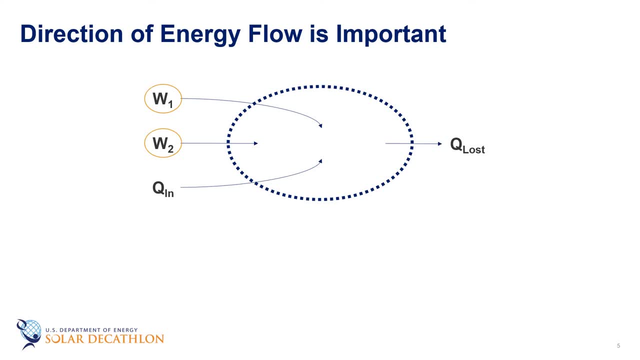 In this case, we have work coming in from two different sources. We're adding some heat from another source and we've got some heat that is lost, And so the sum of these flows is equal to the change of energy, or delta E. Now it's important to keep track of these signs. 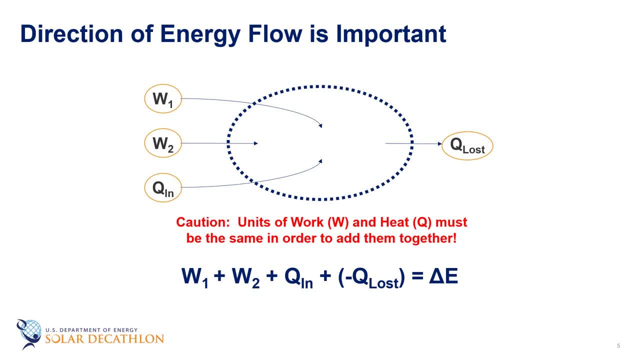 I like to keep everything going in as positive and everything going out as negative. Now, often when we talk about energy flows in and around buildings, we refer to it as something that's happening over a long period of time. Perhaps we are looking at energy flows over the course of a day, a month or, more typically, a year. 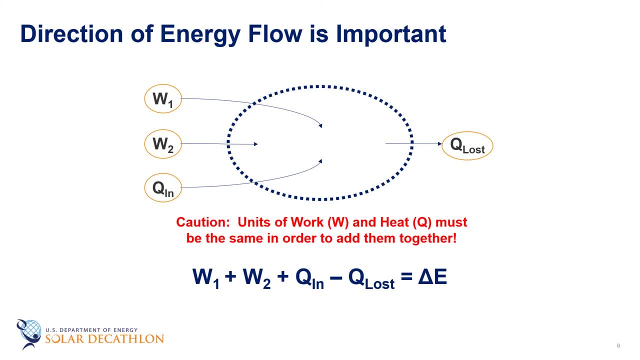 We can think about that building as being in the same energy state at the end of this time period as it was at the beginning, which tells us that the energy of the system does not change over the course of the time period, So that change in E is often equal to zero. 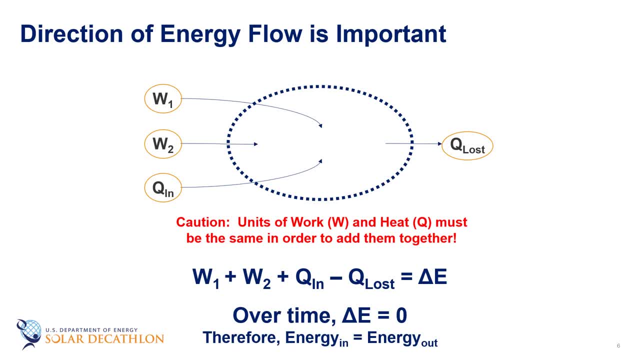 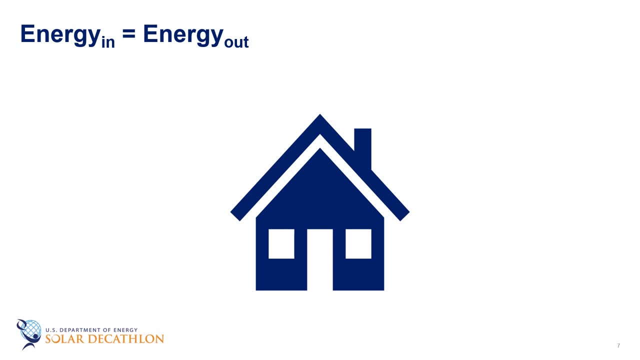 And, at the end of the day, really what we're going to try to do is add up all the energy that's flowing into the building and equate it to all the energy that's leaving the building. So how do we apply this concept of energy in equals energy out, as it relates to building science? 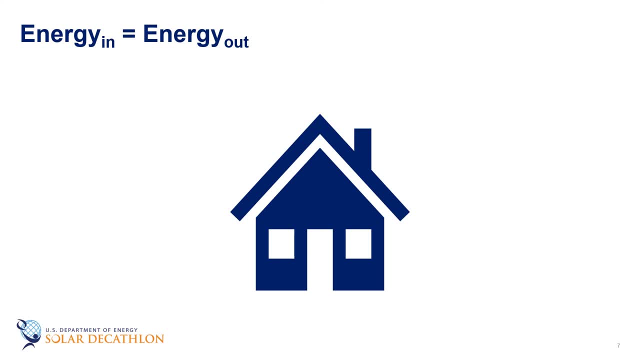 That's actually a very powerful question, because energy can't be created or destroyed, And so then we start thinking: how am I going to measure all of these energy flows? Some of the energy flows are really easy to measure If we have electricity that's entering the house and electricity is technically considered work. 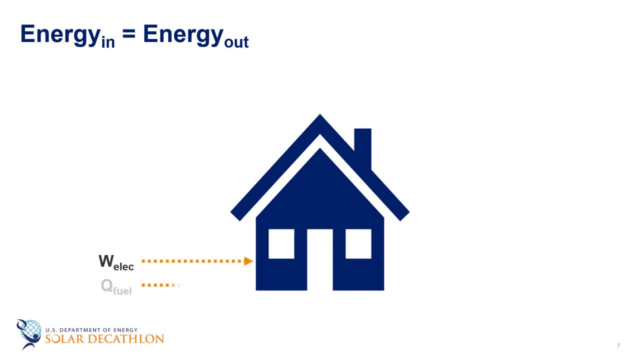 or perhaps we have some fuel that's coming in. we measure those with the utility meter, because that's what we buy. Let's look at a house. Even though we picked a house for discussion, the same principles apply for commercial buildings Such as schools as well.